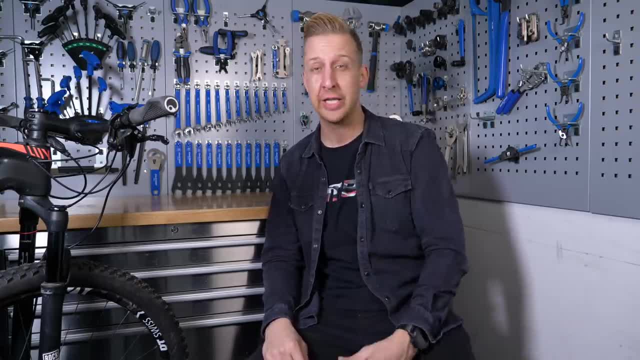 If you're in a workshop and you're in bare feet, flip flops, even just in your socks, you're asking for trouble. really, Bikes have heavy components on them. They've got heavy tools that you start using, things like hammers. 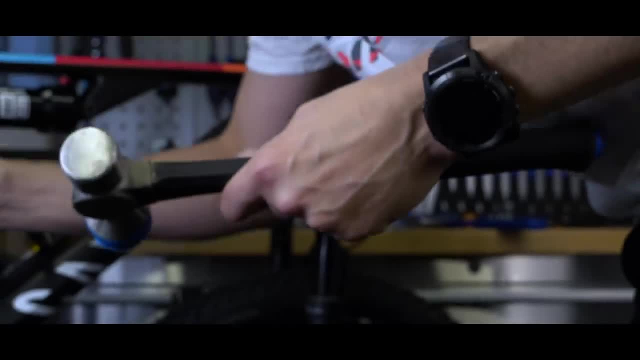 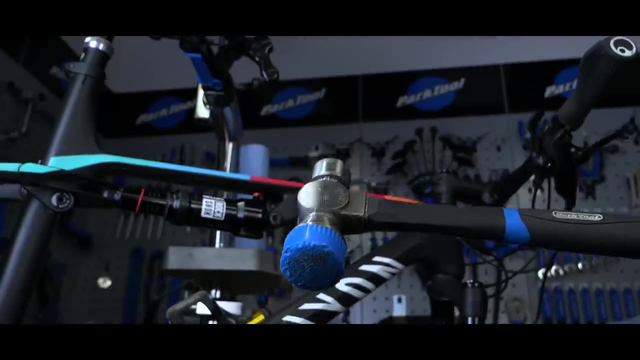 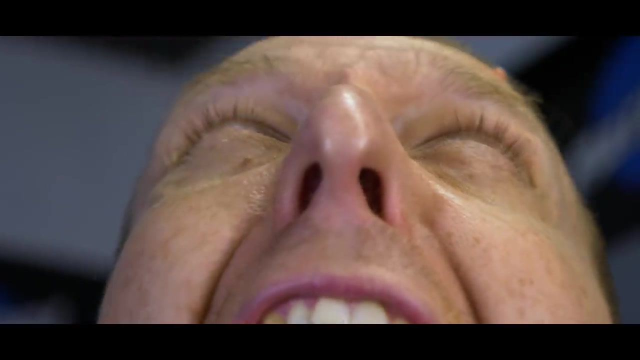 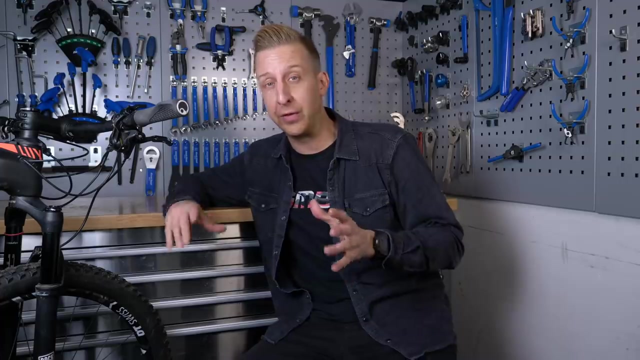 All it's gonna take is to accidentally slip and you're gonna be in a realm of pain. Fettling with your bike naturally means that from time to time you're gonna drop a few things That could be the Allen key set you're working with. 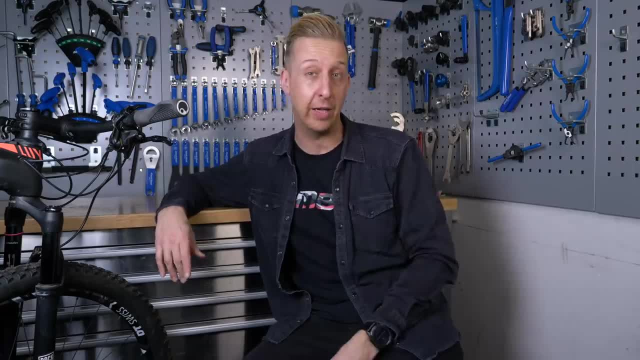 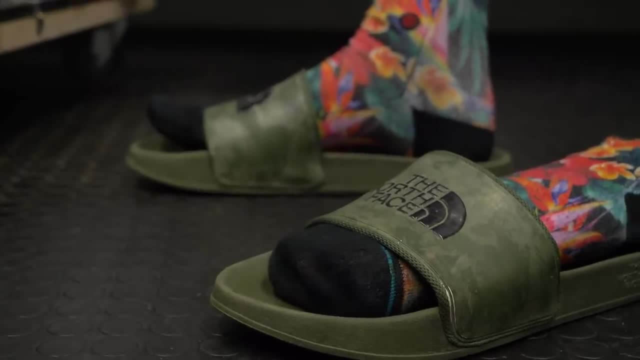 it could be a few annoying washers, or it could be something heavy like a hammer, And I can tell you first hand dropping a hammer on the top of your foot is one of the most painful things you'll ever do. It's right up there with treading barefooted on Lego. 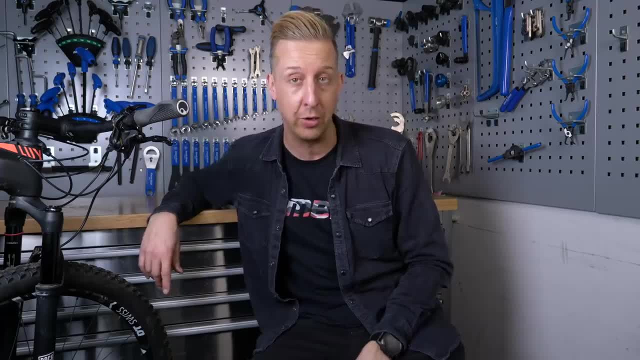 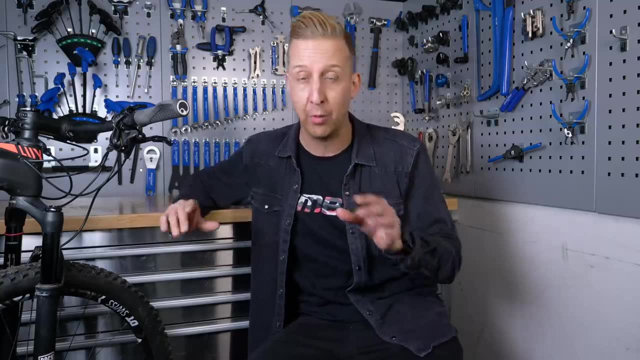 or, even worse, on a plug on the middle of the night when you're on your way to the loo. I can tell you it is exactly three times more painful, 13 times more painful than falling off your bike. But on a more serious note, you are working with bikes. 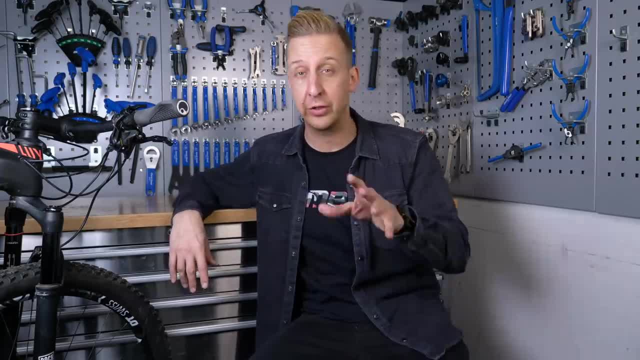 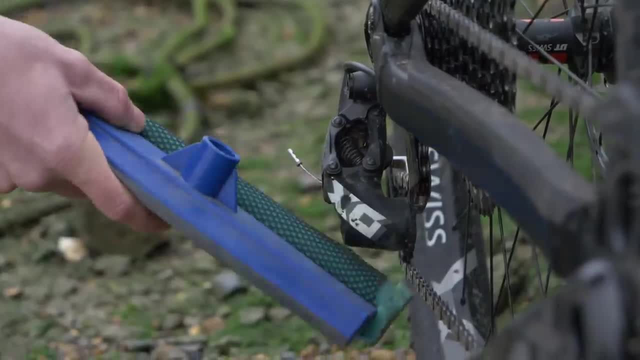 you're working with tools that are sharp things floating around in the workshop, so do take care White T-shirts and light clothing. Bikes are dirty, Drive trains. they're even more dirty Now, despite what those 50 to one boys are doing. 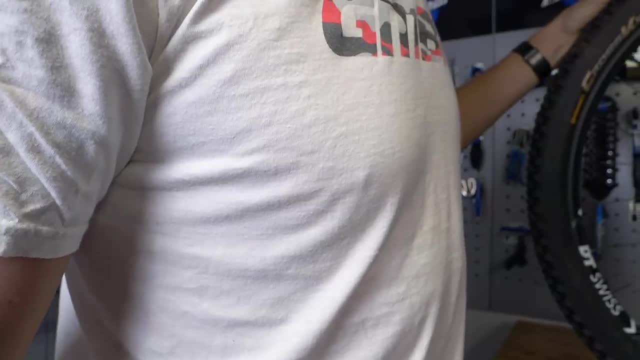 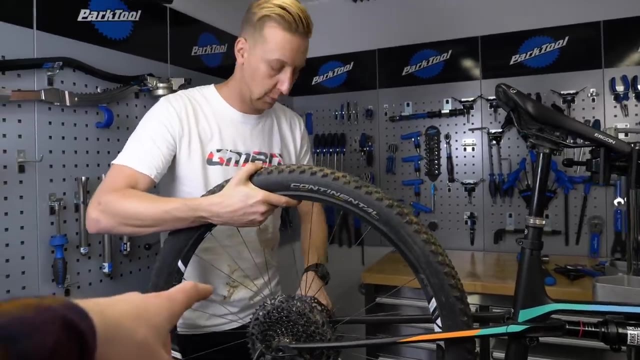 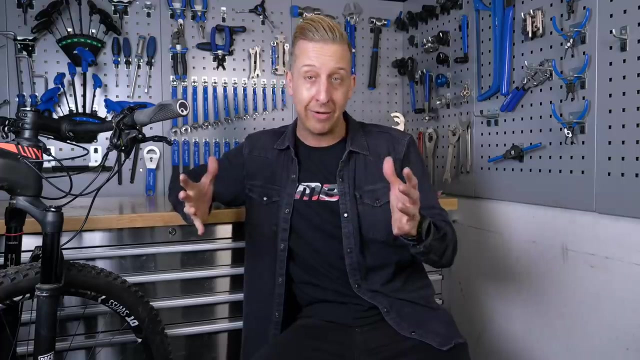 and what all the cool kids are doing. white T-shirts are a terrible idea for mountain bikers, especially in the workshop. Dolly, you're so dirty. look at you. What, what are you talking about? You state Now, wearing dark clothes obviously is a much better idea. 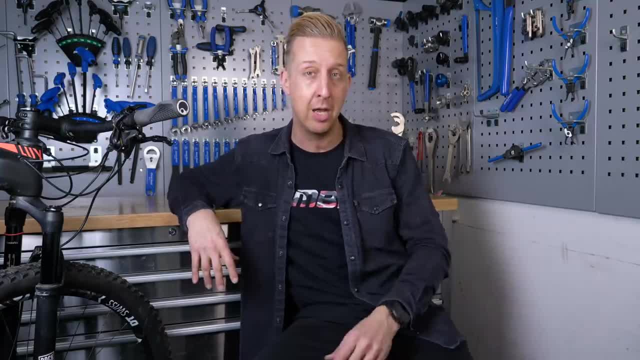 When you do get dirty, at least you can't see it and it means it's easier to wash out. But a better idea is actually just to get yourself a workshop apron. Make a lot of sense. you can stick your tools in them. 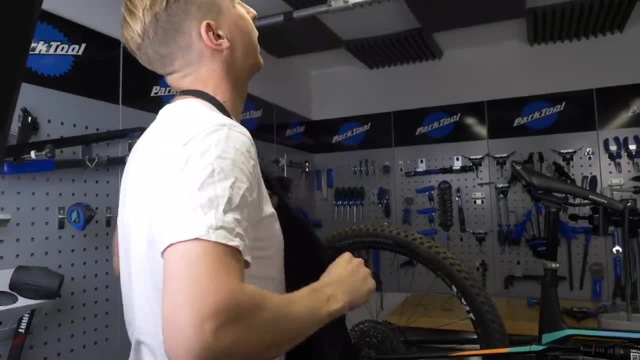 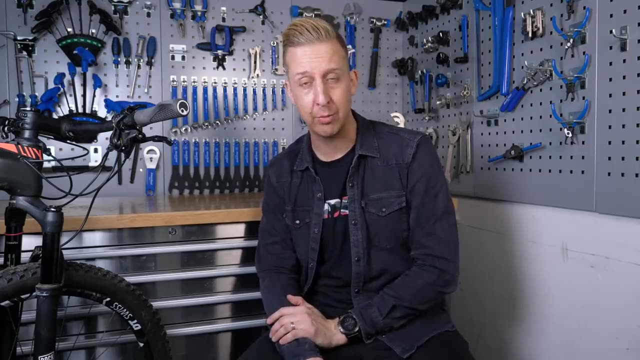 Job done. Give me that Blunt cable cutters. Now, this is a classic workshop error. I see this a lot with people that skimp on cable cutters. They get themselves a nice value set that never really cut through the cable. 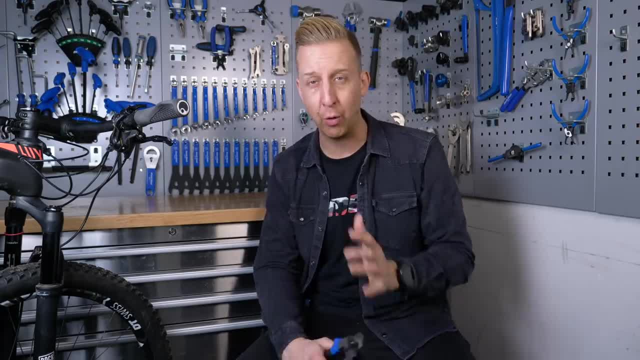 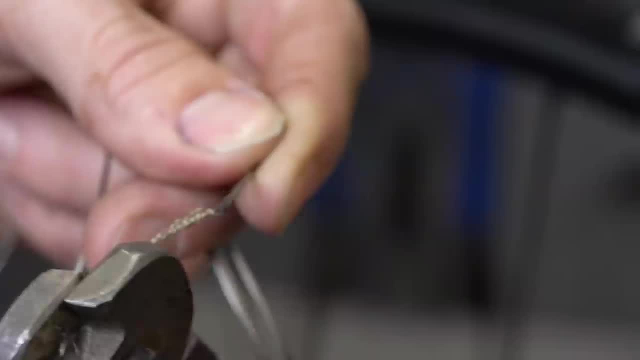 And I see these people like hacking at cables trying to get through. But what you need is a quality set of cable cutters. These will cut through your cable precisely every single time. You won't get any of those frayed cables which cut the ends of your fingers. 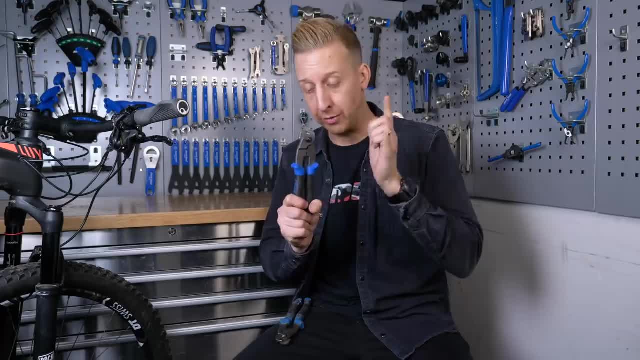 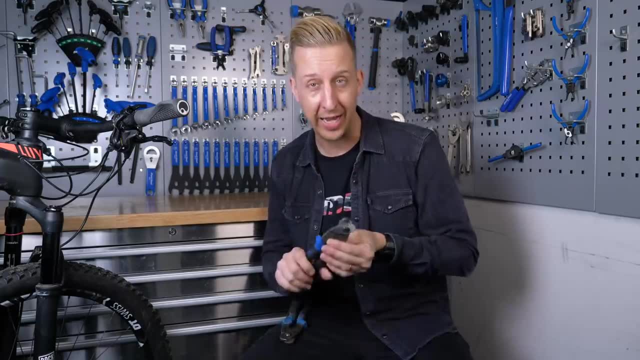 which is excruciatingly painful. One note, though: get yourself a pair of cable cutters. Buy once, Do it right and they will last you, But make sure you do not use them for anything except cutting through cables. Now I've got a really, really old set. 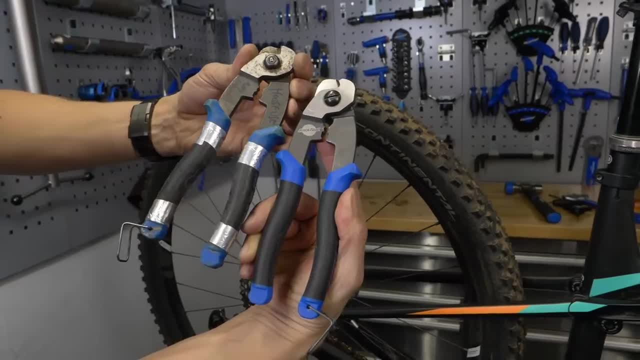 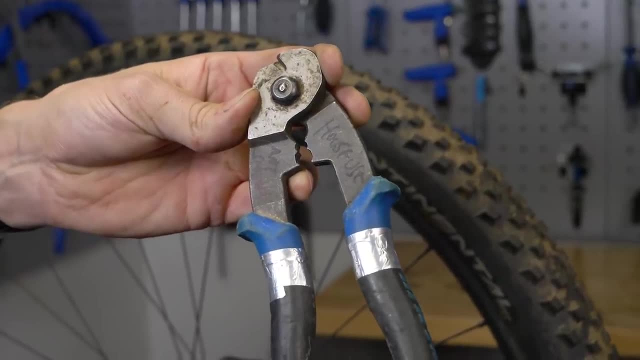 You can see how old and faded they are by comparison to these brand new workshop spec ones. These ones are now retired from use as cable cutters and I use these as generic cutters for cutting cable ties, cutting through spokes, anything like that. 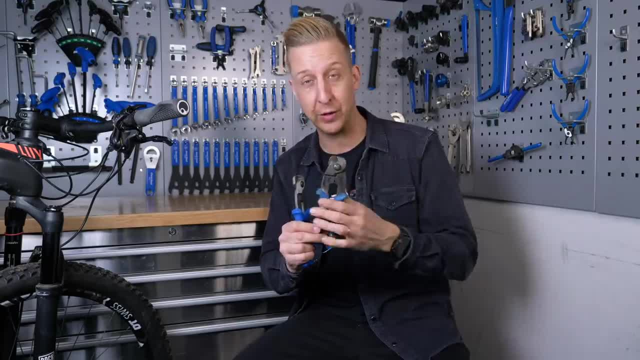 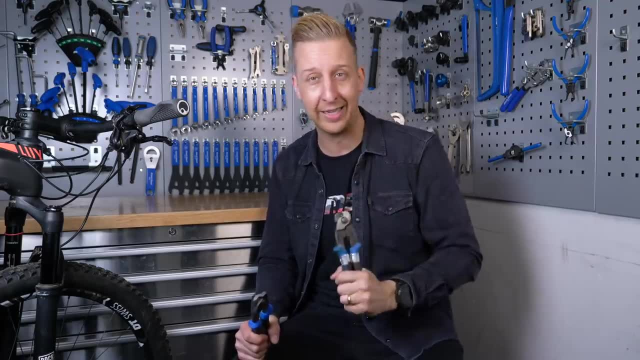 And I've marked them up with some silver tape, so I know that these are no good for using on the bike. I definitely recommend doing the same if you've got a knack of a pair, because you can still get use out of them. Just don't go hacking at your cables. 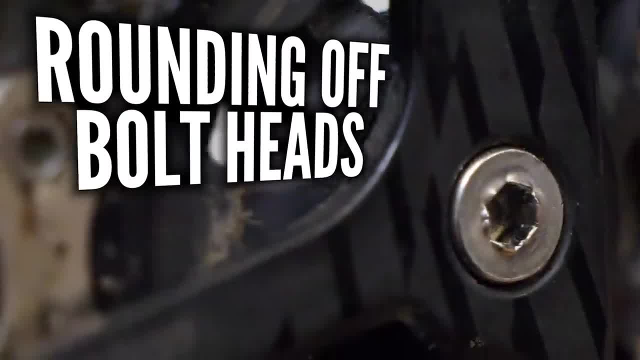 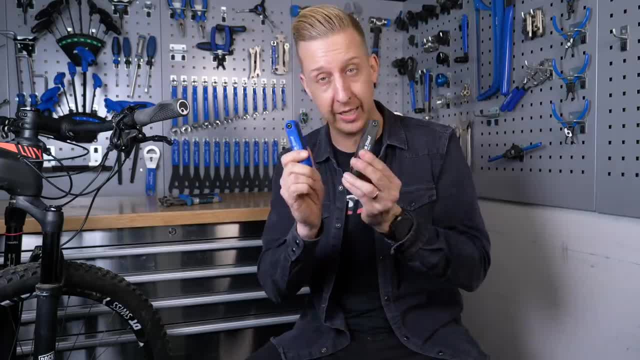 Get yourself a nice, fresh, sharp pair and only use them for that: Rounding off bolt heads. Now, possibly one of the quickest way to round off a bolt head is getting imperial and metric allen keys confused Now, thankfully in the mountain bike world, and the same in the road world. 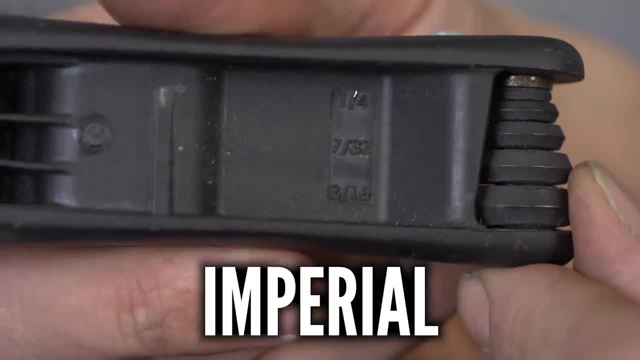 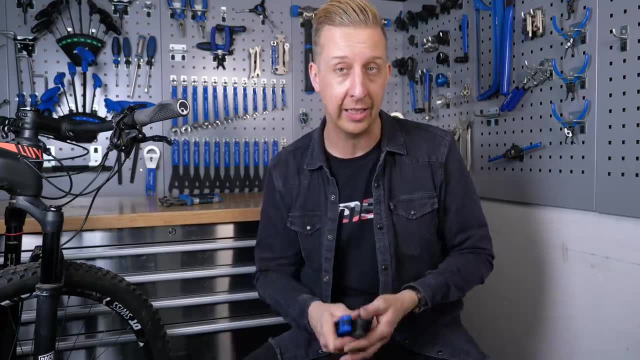 you don't really see a mix of imperial and metric these days. Really, you do see some of that in the BMX world and of course, you'll see it from other sports. So if you've got a toolkit that has varying allen keys, make sure you keep them separate. 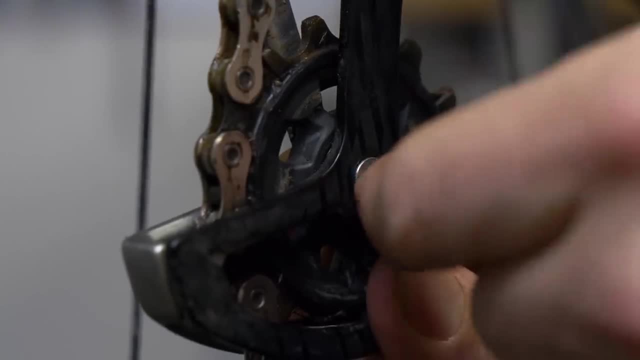 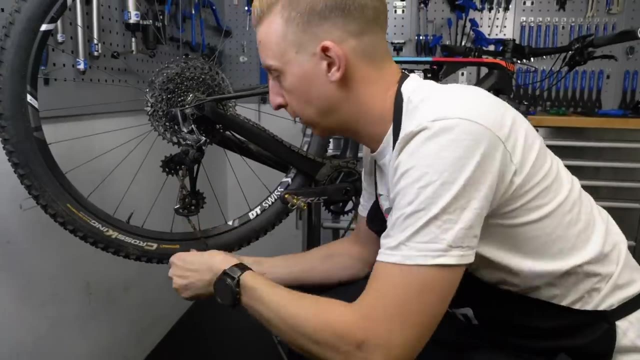 because it can be really easy to find one that looks like a five or looks like a four. jam it in the bolt and round the head off. That is not good. Just need to sort this jockey wheel bolt Three mil. Thank you. 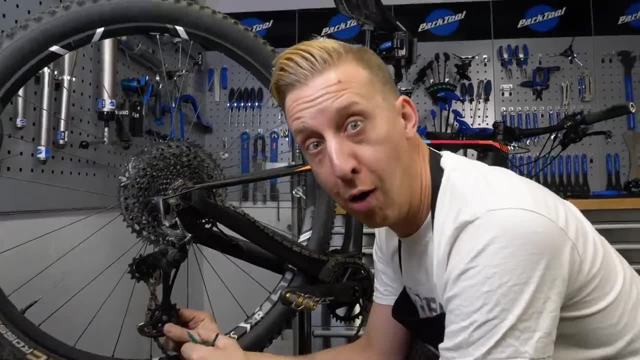 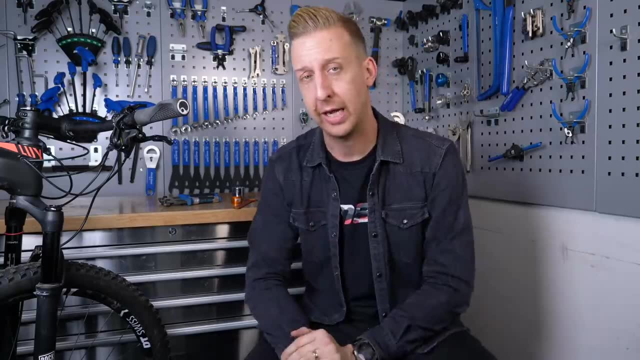 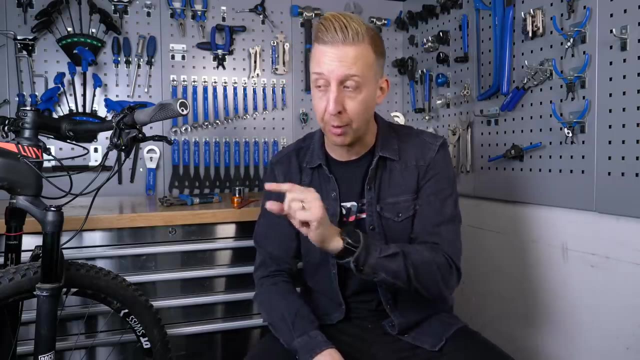 There we go. Oh shit, Mano and SRAM rear. derailleurs, both have tiny little counter sunk bolts that hold the jockey wheels in place. Now, these are super easy to use. You just need to round off. So make sure that A the bolt is in vaguely good condition. 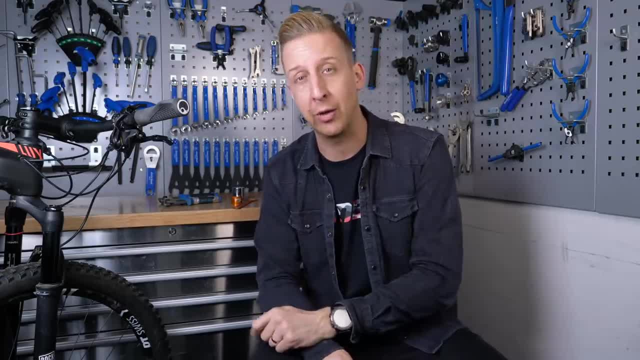 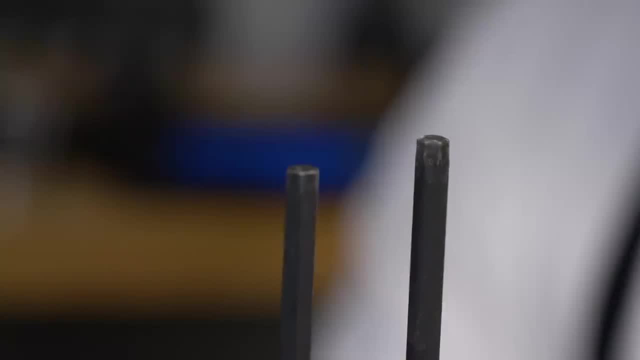 before you even start using it. B make sure that your allen key is in fine condition. It's got nice sharp chiseled edges on it. Don't go using an old one that's slightly rounded. You're asking for trouble and it's going to be a big pain in the ass. 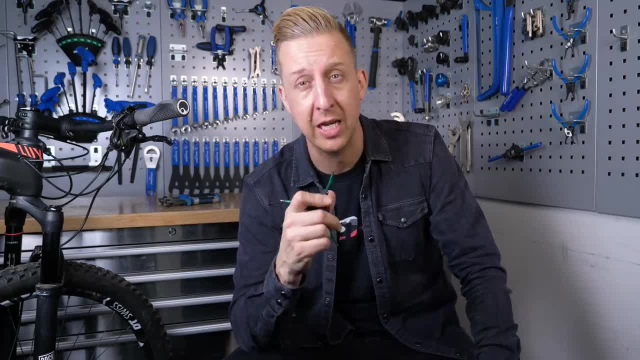 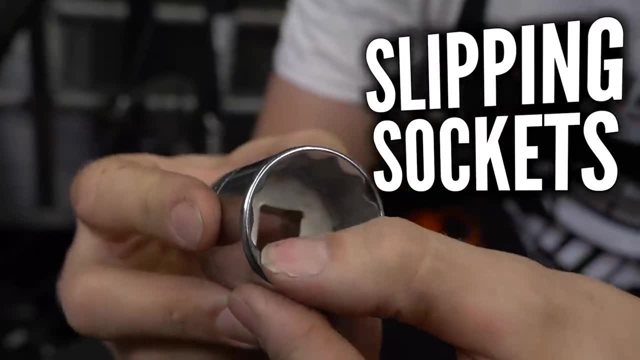 And ultimately, this is why we tell people to buy quality tools: because they last a lot longer. Remember the motto: Only a rich man buys cheap tools. Slipping sockets Now the top cap on most of the bikes, most suspension forks. you will need to access this. 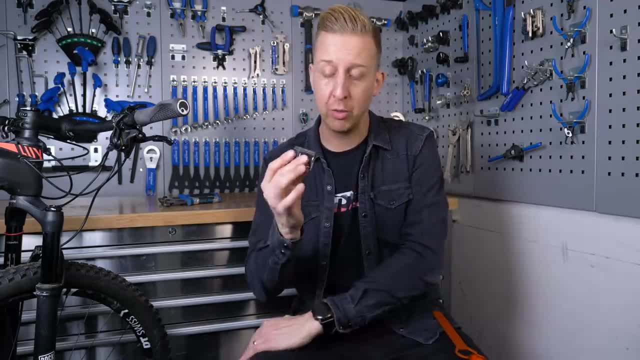 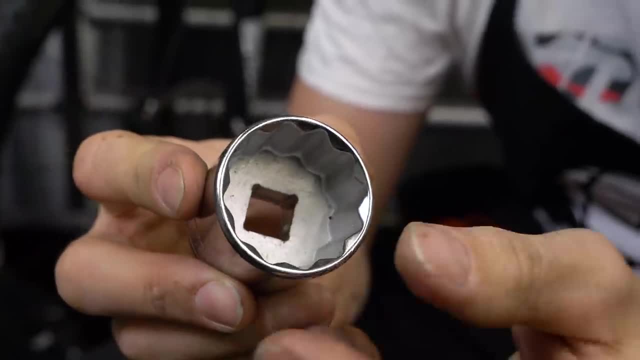 in order to put air volume spacers in. Now you'll think a normal socket is the ideal thing for this, but most typical sockets you'll get in tool kits will have slightly chamfered edges, like this one here. That's to aid them, to get them to slide. 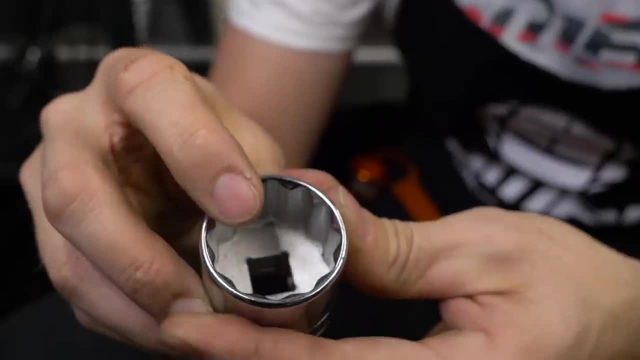 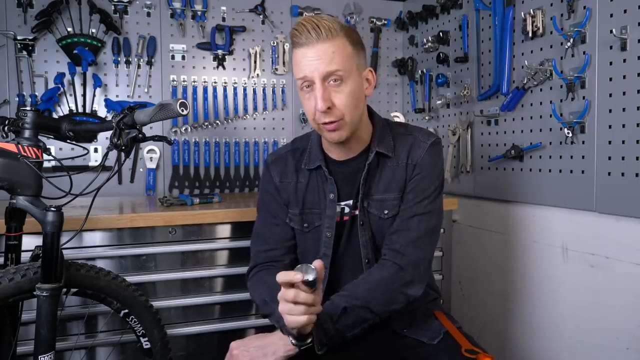 onto a bolt head nicely, But in the case of a real shallow headed bolt head, like you see on the top of a suspension fork, this is a really, really bad idea. They're made of soft aluminum and it does mean that you're actually round those edges off. 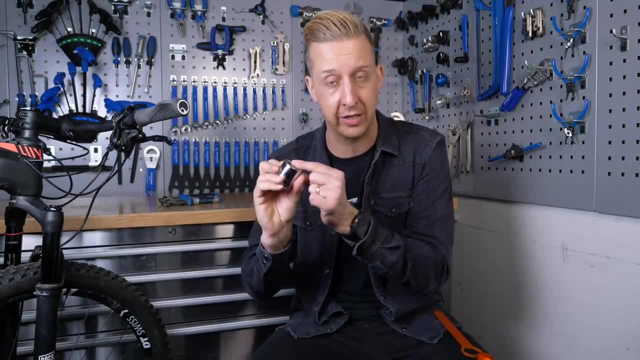 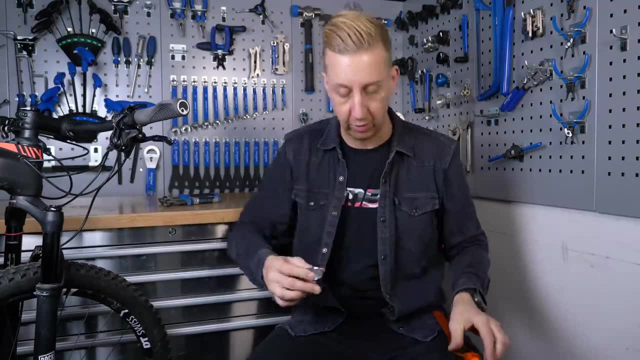 Really fast. so don't use one that's got edges like this. What you really want to be doing is either get yourself one that's already got a flat surface to it, get an old socket and grind it down, or get yourself a purpose built one like this one. 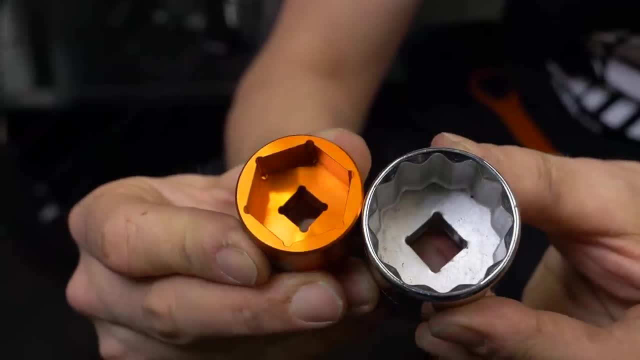 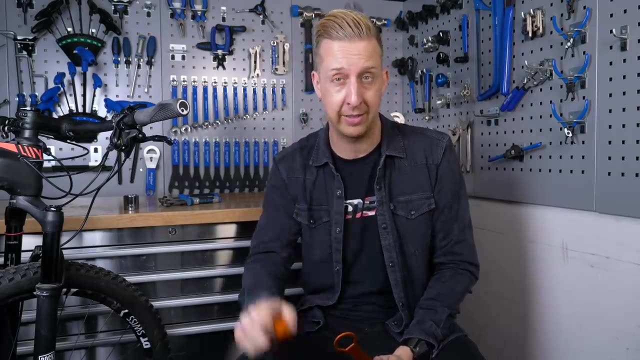 for example from Fox, designed for the fork, and you can get purpose made spanners exactly for the job. And if something like this is the sort of tool that you're not going to use that often, chip in with your mates and get a set between you. 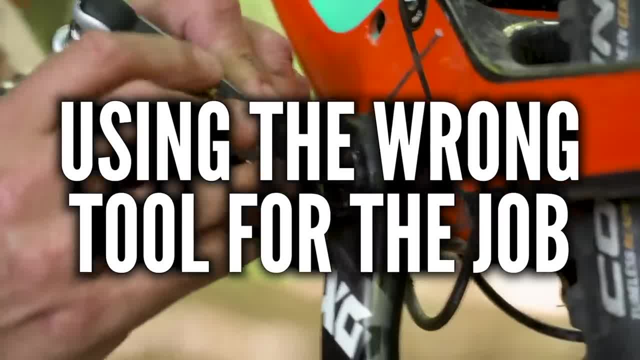 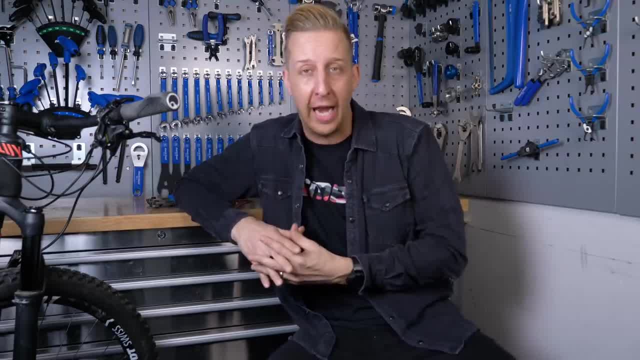 of those less commonly used tools. Well worth it Using the wrong tool, The tool for the job. Now, I think we all know where I stand on this. I think that you should have the correct tools for any job. It doesn't always happen like that, and it does mean. 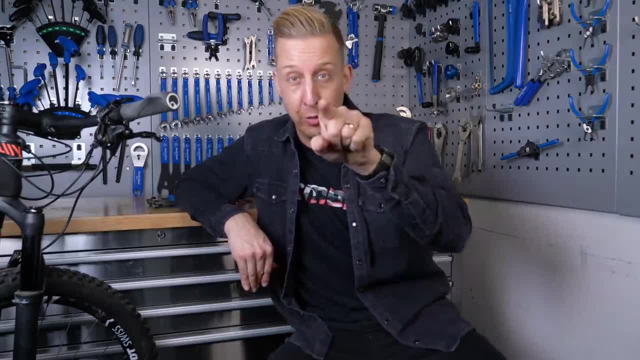 that a lot of the time. you see people bodging. Yeah you, I've seen you doing it. I've done it from time to time and I've got to say it is quite useful to be able to bodge here and now. 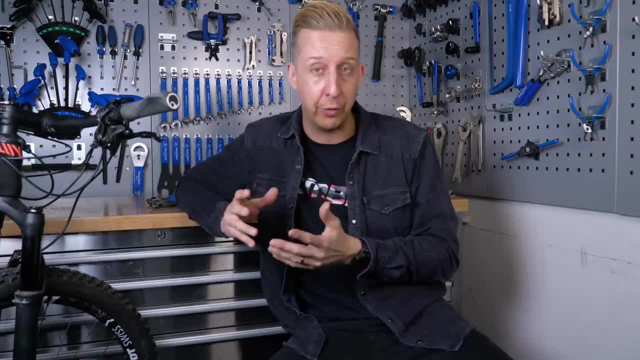 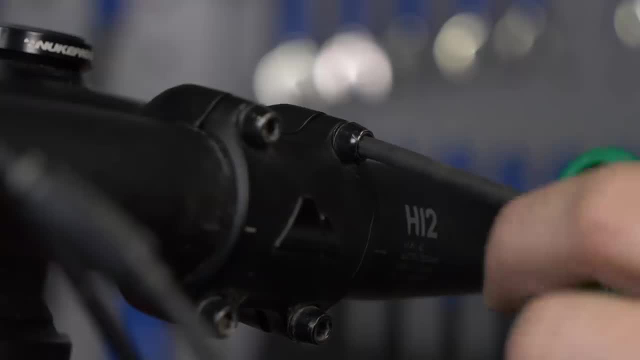 What I'm talking about is if you do find yourself in a situation where you round off the head of a bolt- say it's a four millimeter one on the front of a stem. you can actually sometimes get a T25 Torx key into that. 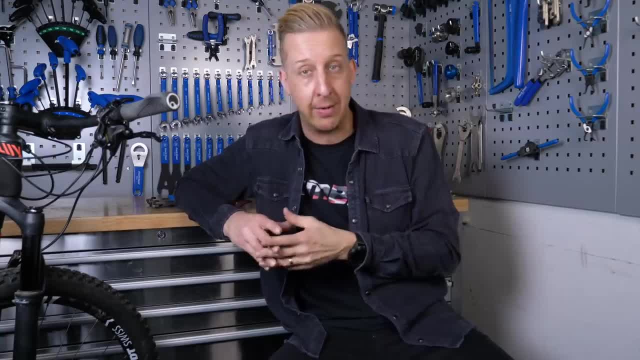 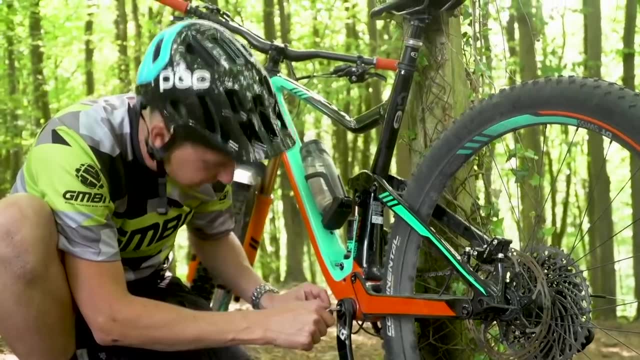 It will find some traction. so sometimes it can be useful to sort of get you out of danger. And likewise, if you're at the side of the trail and say the eight mil bolt on your crank has come loose, you can wedge a six and a two in there. 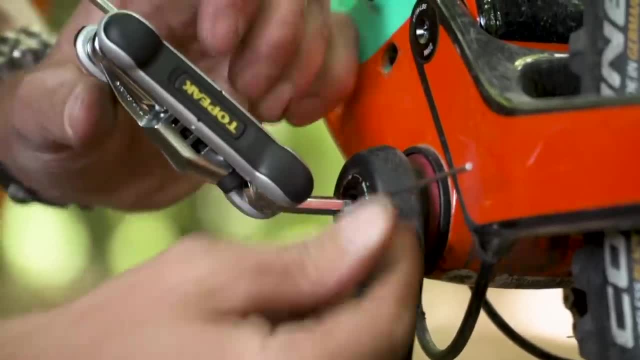 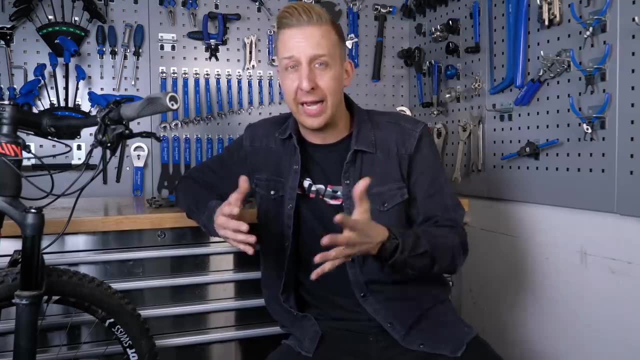 and it will just about nip it up tight enough certainly to hopefully get you to the next spot, or until you find another rider that will have an eight millimeter. And well, we've all done it. We've all fitted a headset with a block of wood. 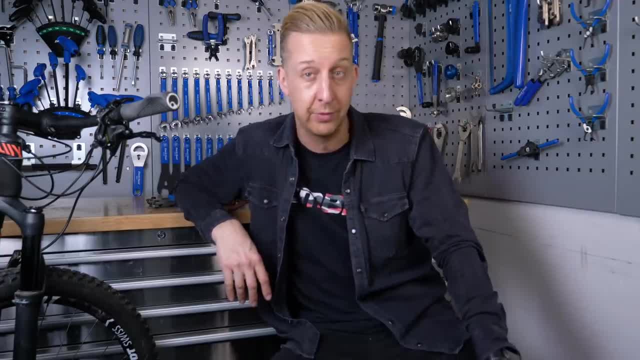 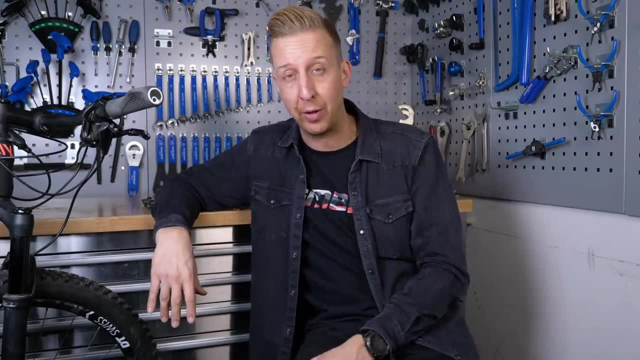 and a mallet, but that's for another video on GMBN Tech soon. Just keep an eye out for that one. Being ham-fisted: Now we've all seen this one. There's no excuse for it. Being ham-fisted around a bike. 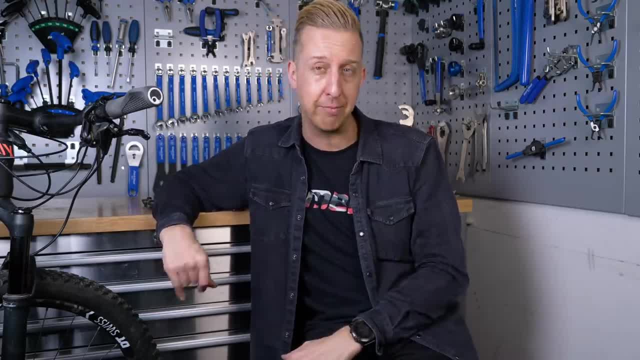 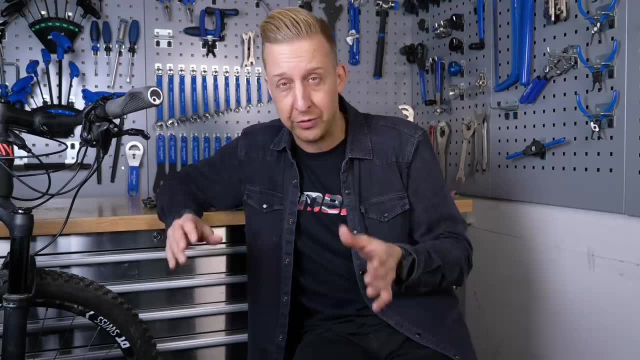 isn't going to get you anywhere And, if anything, it's just going to cost you money. Now, working on bikes isn't hard As long as you follow a procedure. it's pretty logical, to be honest. So just take your time. 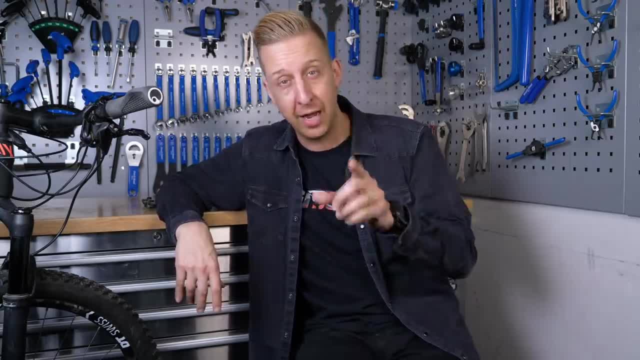 If there's a job that's frustrating, you walk away from it. Get a bit of fresh air. Never work on a bike when you're in a bit of a mood. your stress level's pretty high. It's never going to work out that well. 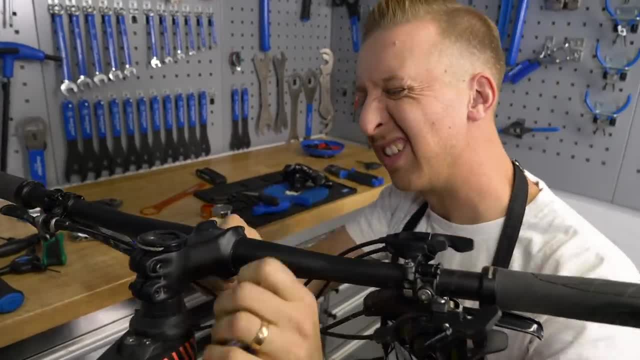 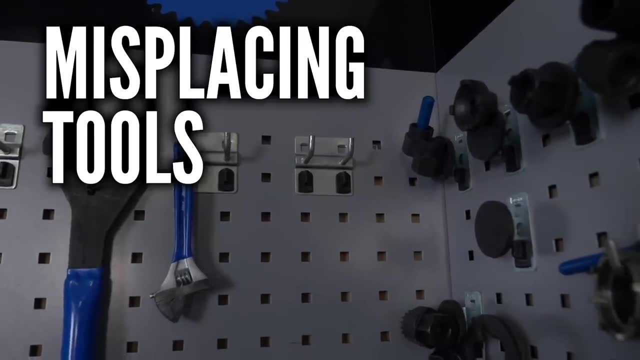 All you're going to end up doing is snapping a bolt, rounding a bolt off, or doing something you're really going to regret, especially in the wallet department: Misplacing tools. The main answer to misplaced tools are lending them out. Do not ever lend your tools to anyone. 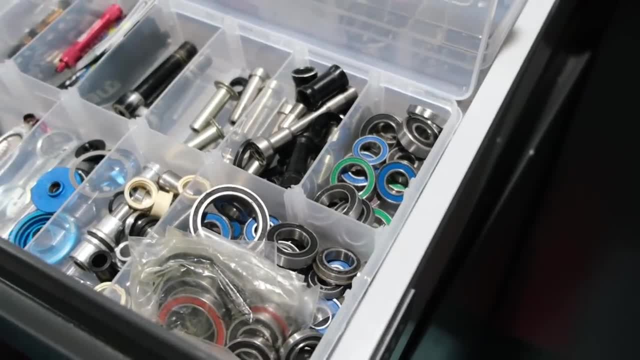 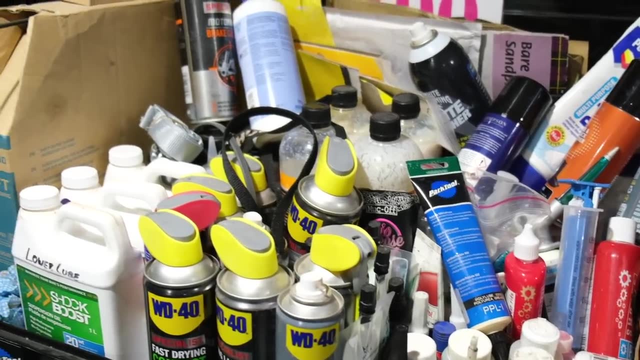 because you won't see them again. Now every tool needs to have a home. Now you don't have to have a workshop quite as well organized as this place or even as retentive as my own workshop, which is pretty retentive, to be fair. 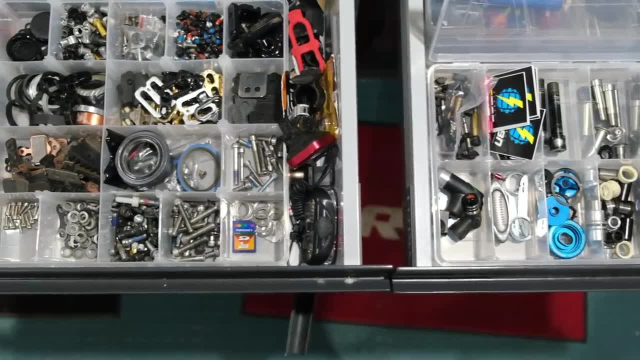 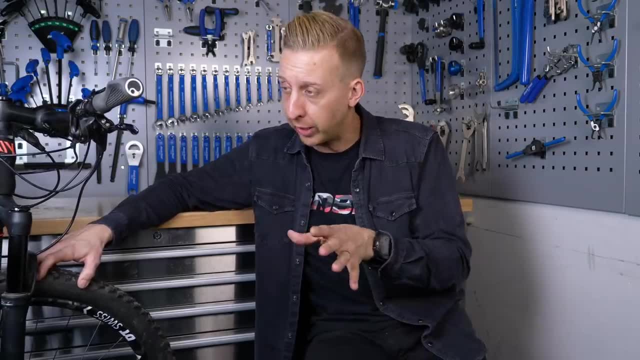 But it is important that you do have somewhere to store your tools. You do that and you're going to be able to avoid the rare phenomenon known as workshop rage. Now, this happens when you're working on your bike. you're just about to go out riding. 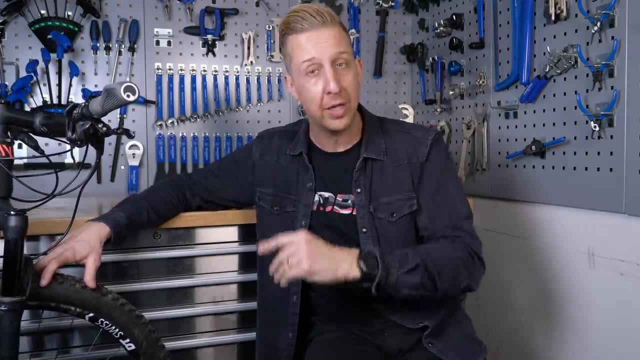 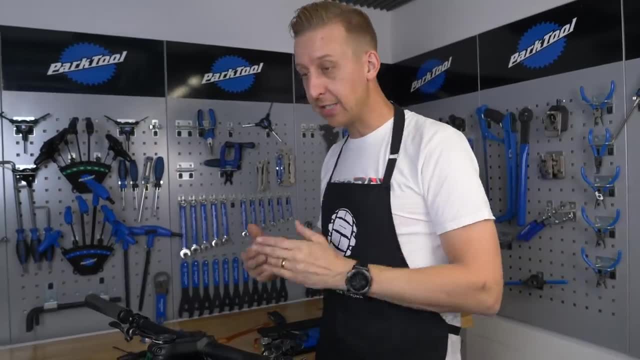 and there's one crucial tool missing that you need. It's always something like a five millimeter Allen key, the most common thing there is. Where is it? Yeah, you lent it to a mate, didn't you Cool? and the last thing I need is just a mallet. 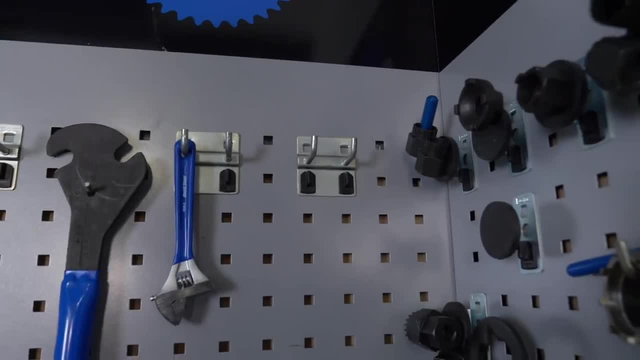 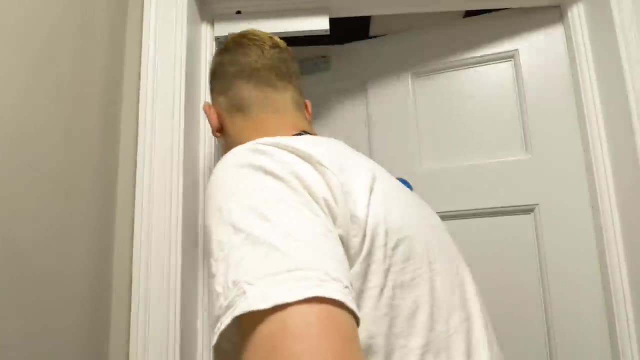 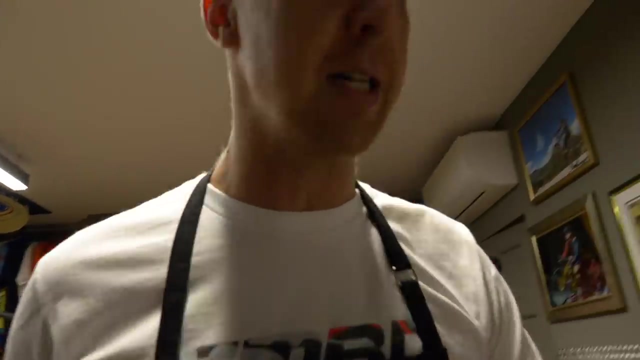 just a seriously. It's got one place. I bet those guys next door to GCN, I bet they've got it. Oh, there, it is Nice flipping roadies you've been using for anyway- Probably can't even pick the thing up. 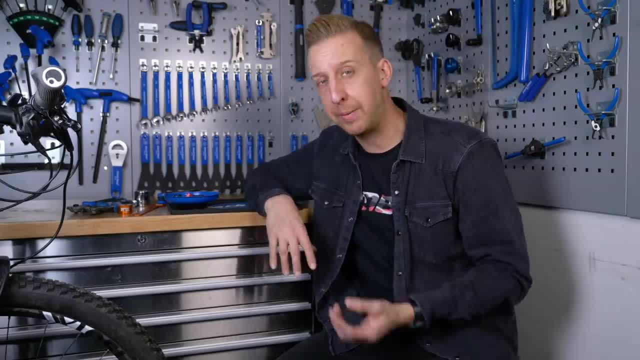 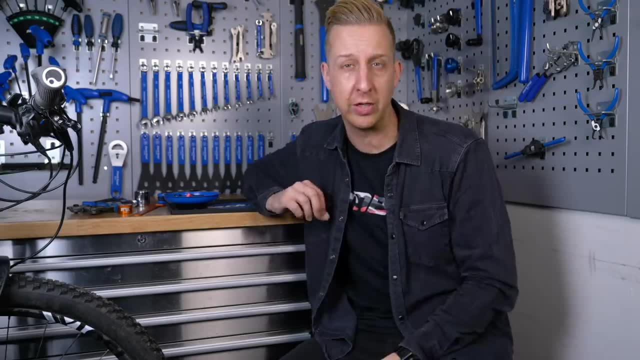 Misplacing small parts. Now we've all done this before when we've been working on bikes. We've dropped stuff, it's flown under the fridge or wherever it's gone. It can be so annoying and it can be right in front of your eyes half the time. 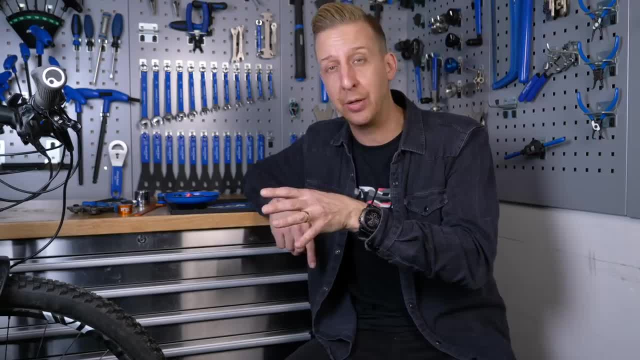 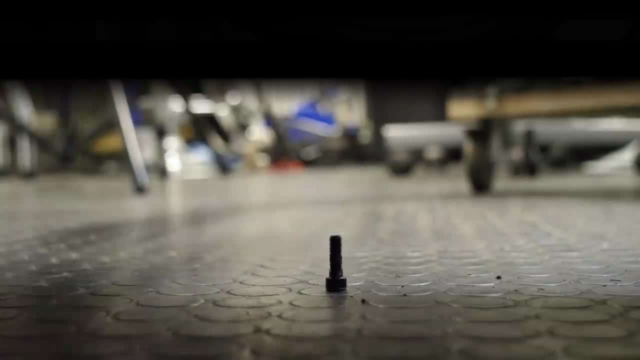 You waste time trying to find this stuff Now. it will always happen, even before, when you're preparing to go for a ride. you need to get an early night's sleep in order to get up and ride all day, or just before you go riding. 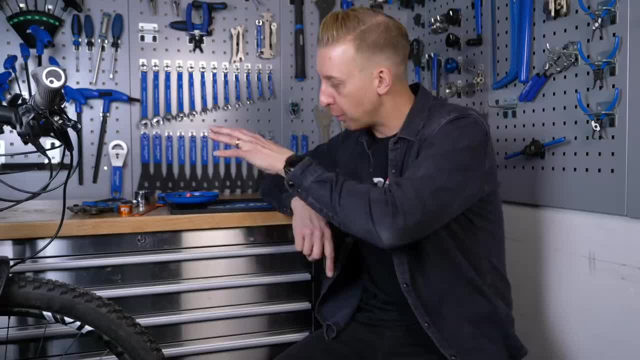 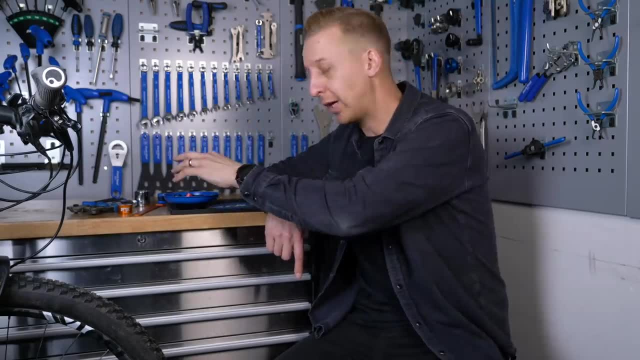 in which case you're wasting valuable riding time. Now, having some sort of magnetic parts tray, that's a great idea, because you can just, for example, lock on grip bolts, stuff like that. You can pop them straight in there. 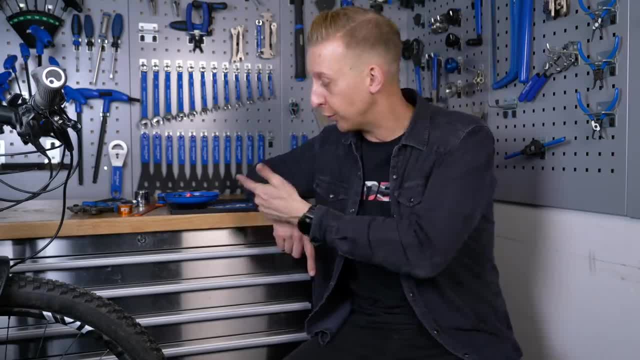 They're going to stick in there, Not going to go anywhere. You're not going to lose them. You can even drop these things, and it's so magnetic that the stuff doesn't really fall out. Now, if you're working with a few more parts, 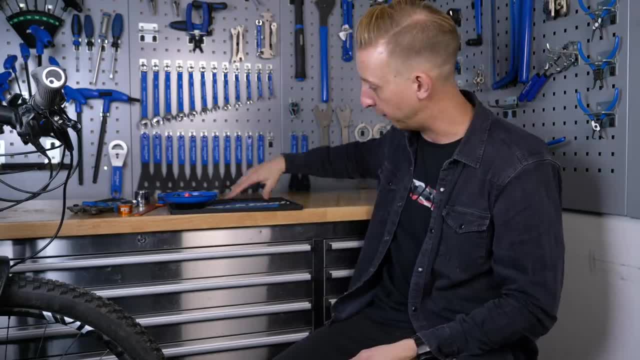 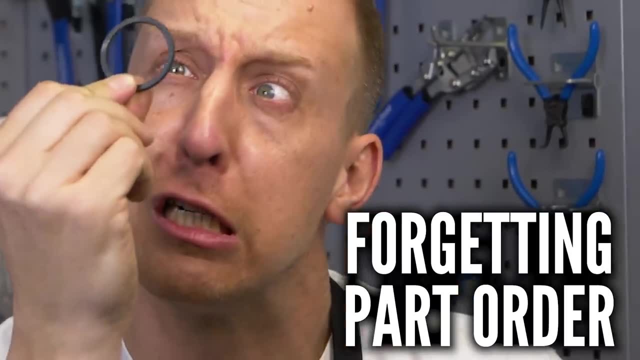 it's worth having a rubber mat on top, on top of your work bench. They have little compartments on the top of them and they're really, really good for just making sure your parts don't go missing, Forgetting the order in which you need. 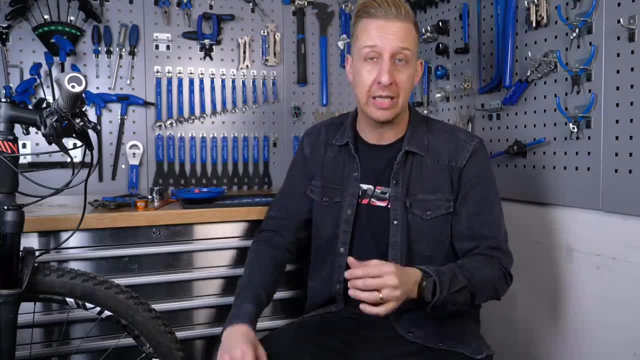 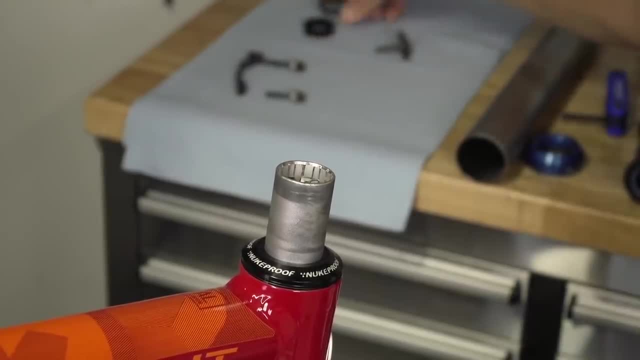 to reassemble parts of your bike. Now, this is an absolute classic and it does directly go on from losing parts and misplacing parts. Whenever you're working on parts of your bike that have multiple components and parts to them, always lay them out on your work bench. 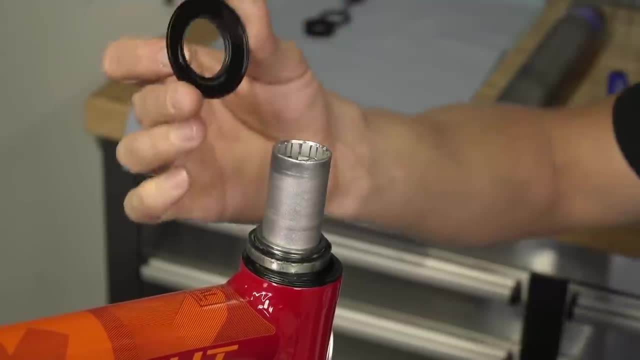 It's a good idea to put them on a rubber mat or some shop towels so they can't roll off and go anywhere, and put them in a reverse order, so you know, when you have to put it back together again, the order in which they go back on the bike. 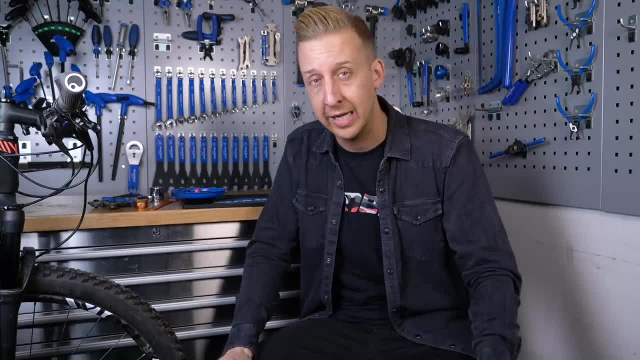 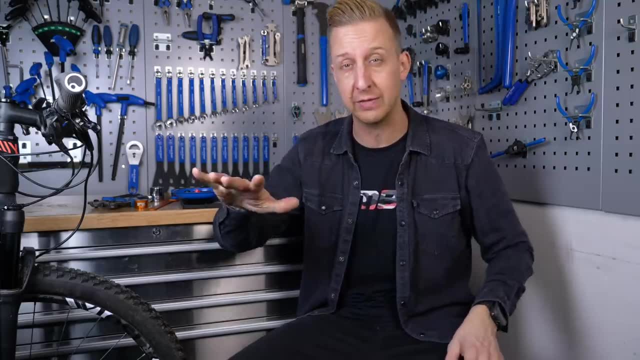 and also you can't have any parts left over afterwards. Now I've seen some people try and reassemble headsets and forks and all sorts of stuff in the past, where they've just chucked the stuff down on a work surface. 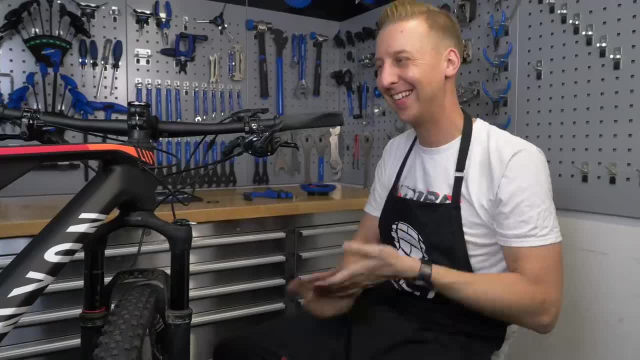 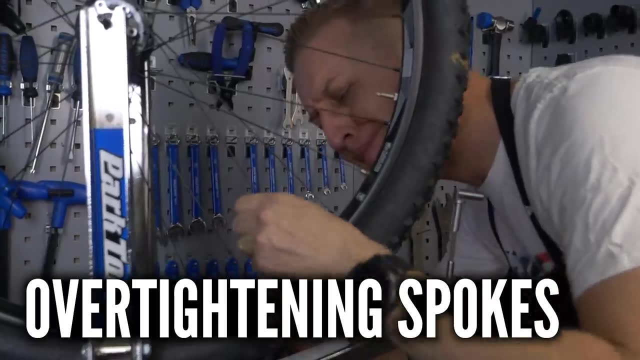 and they're always left with something afterwards. You never want to be in that position, because it might go together okay, but you'll be left with something that's actually quite crucial to the way that your bike works: Overtightening spokes- Now this is another classic. 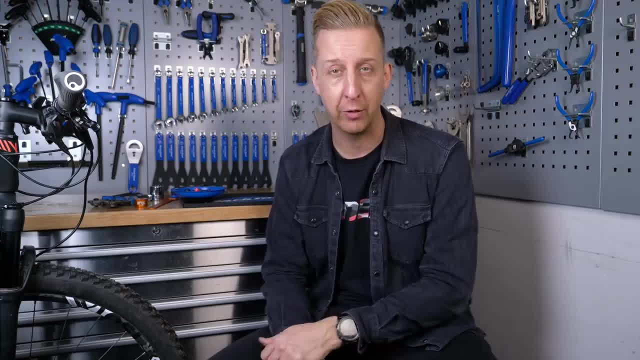 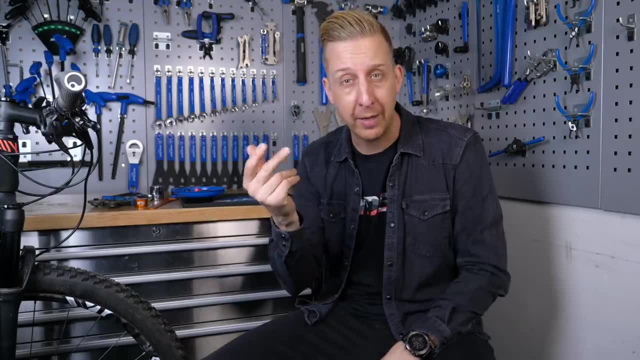 so you've got to lose spokes or your back wheel is a little bit buckled from that downhill run you've just done, so you start attacking it with the spoke key. Now the idea is, if you do have a loose spoke, you just want to nip it up tight. 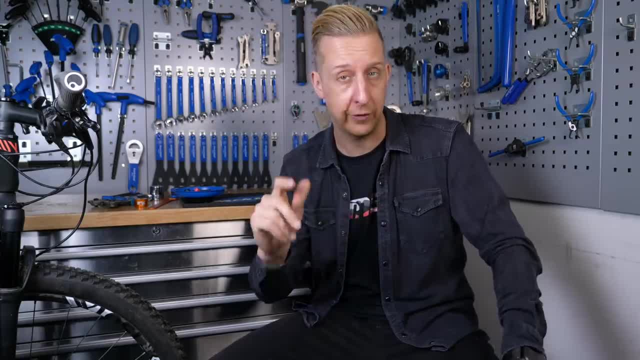 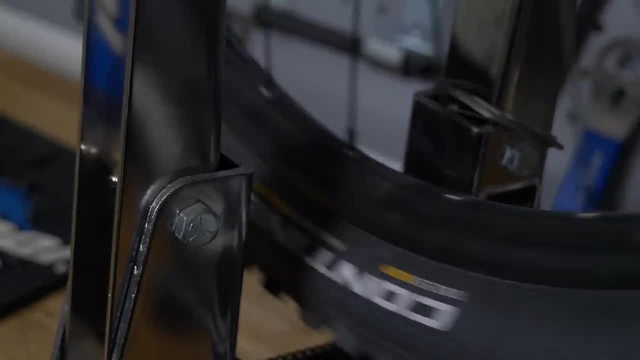 and then start working on it quarter turns, maximum half turns at a time. If you just start cranking away on it until it gets tight A, you're going to ruin your wheel. That's a good way to make your wheel egg-shaped. 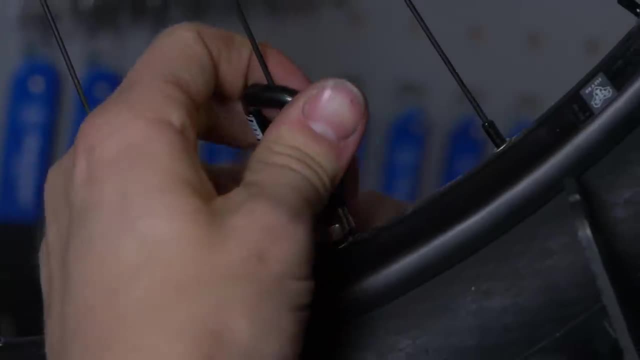 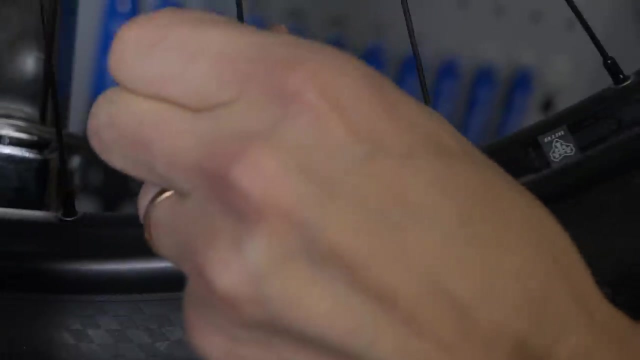 instead of round. and, of course, if they're that tight and you're struggling to tighten them, stop. You need to relieve some of that pressure elsewhere on the wheel. If you just keep tightening, you're going to round off that nipple. 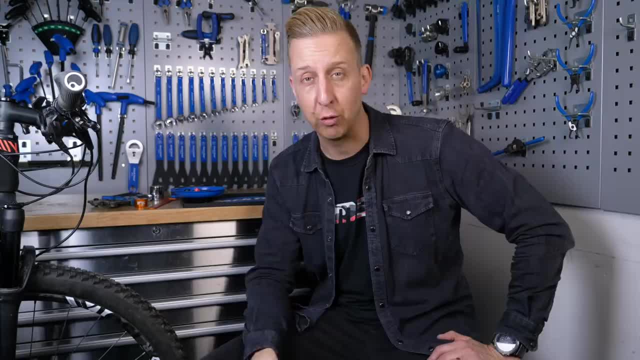 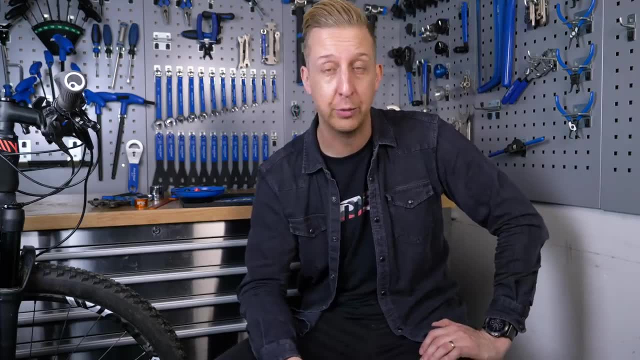 and then the only way to get out is by cutting spokes out. and, of course, if you're not thinking straight, you're going to use your nice posh cable cuts to do that, which is why I always tell you to never overtighten spokes. 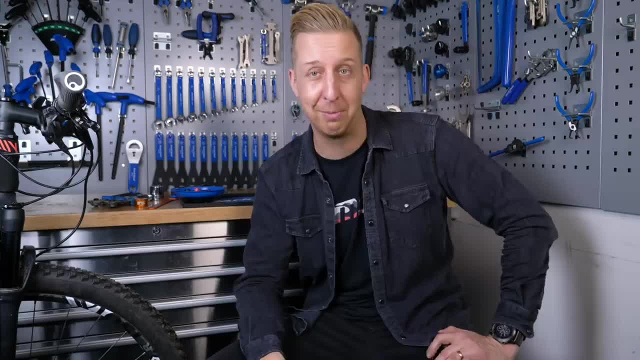 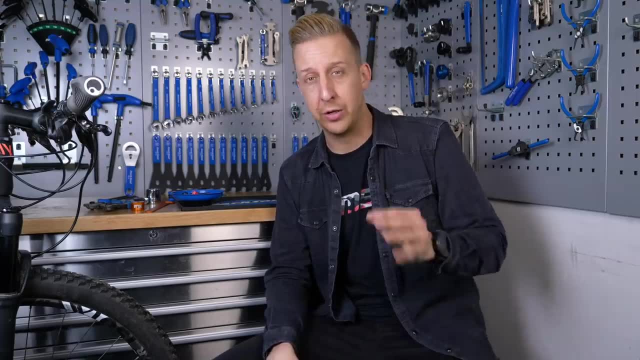 and always keep a set of old cable cuts handy, in case you do overtighten your spokes and you need to cut one Overspraying lubricant. Now, this is something a lot of people are guilty of When you're lubing your chain.